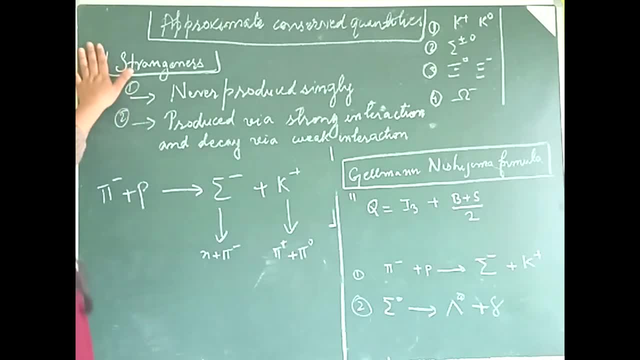 So what is strange about these strangeness particles, right? Or your strangeness quantum number? It is these two things, which is they are not produced singly. You will see here, these two are the strange particles which are being produced, So they are not produced in a single number. Not just sigma minus is not produced singly, or k plus is not produced singly, right. 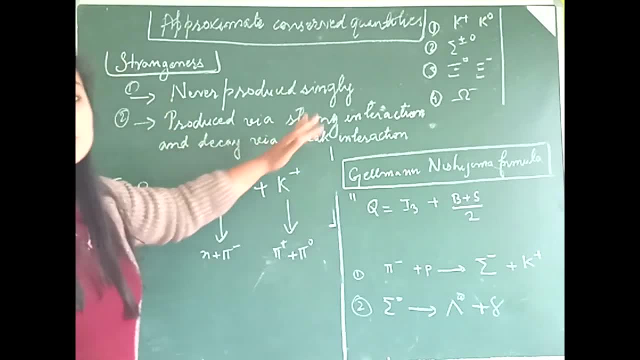 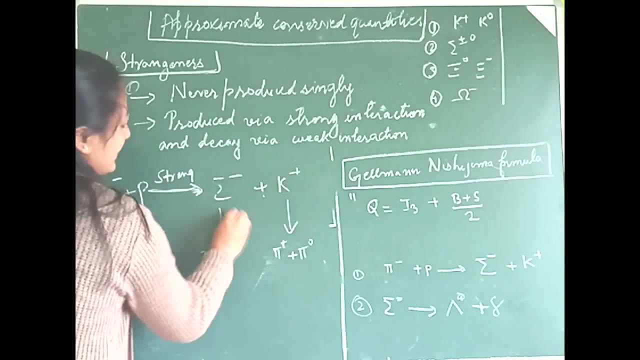 They are produced in pairs. Another one is they are produced via strong interactions. But what is this? When they decay, they decay via weak interactions. So that is your strange quality about this: strangeness particles. So here, they are produced via strong interactions and when they decay, they decay via weak interactions. okay, 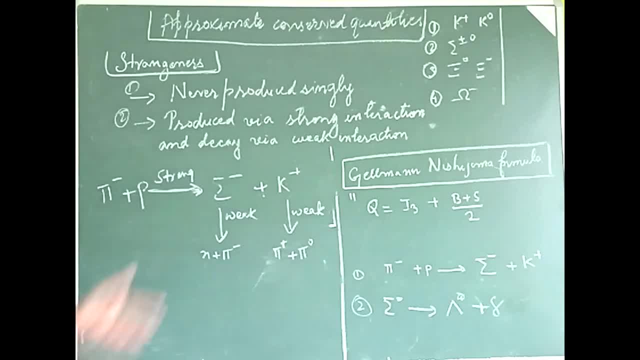 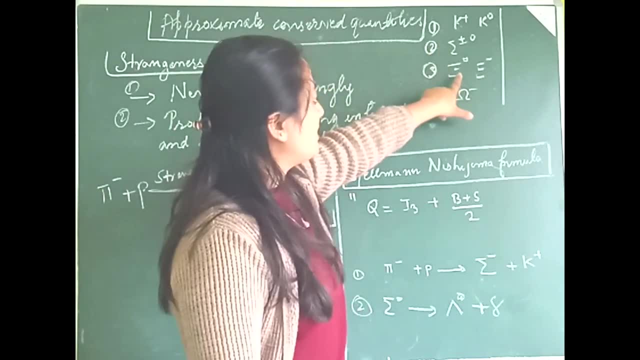 So now, what are the examples of your strangeness particles? So those are your kaons and hyperons, right? So hyperons meaning. so these are the examples of your hyperons. So these are your gemmas, your cascade- this is the symbol for your cascade and your omegas. 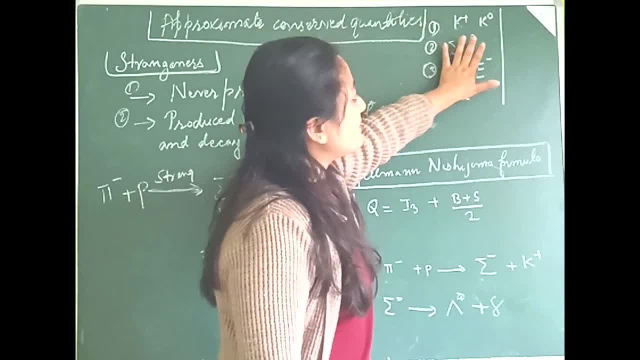 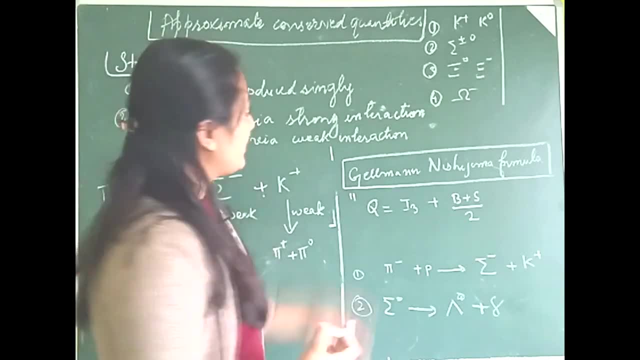 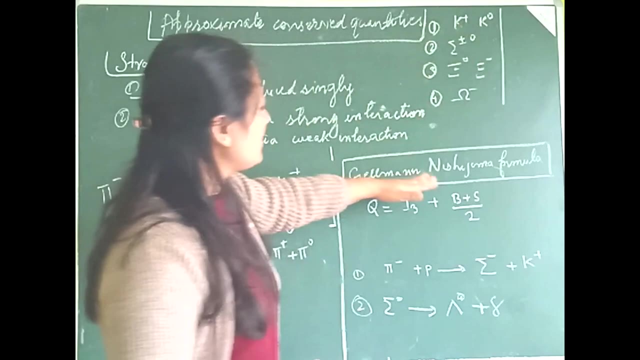 So these are called your hyperons. Hyperons meaning anything, which is the particles which are baryons, but they are little heavier than your nucleons. okay, So now we will be finding the formulas and the strangeness value for these particles by using, by making use of your Gelman-Nisijima formula. 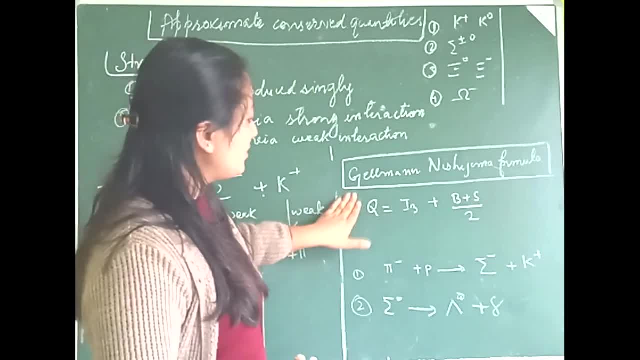 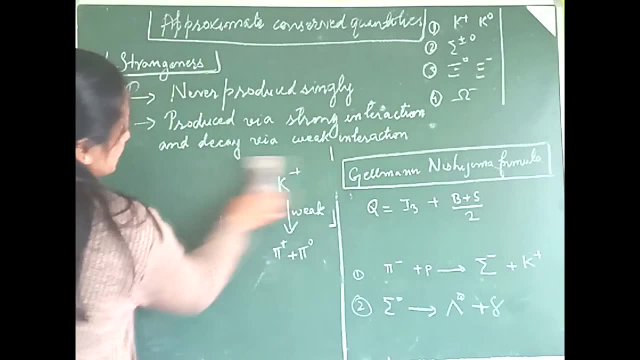 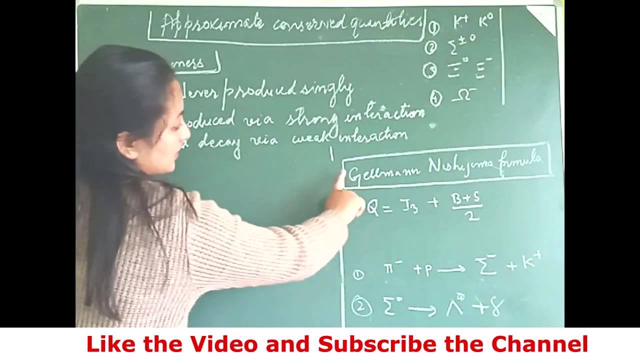 So, according to this formula, you have: your Q equals to I3 plus I2.. I3 plus B plus S by 2, right, Okay? Now, having said that, let me calculate the your S value for these particles. 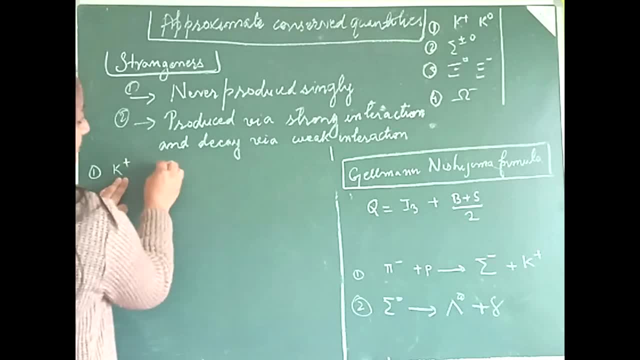 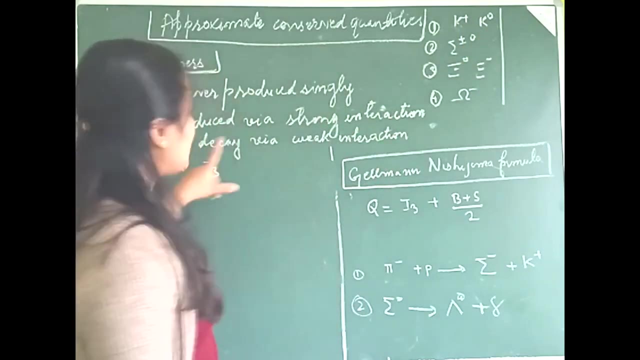 So let me do it one by one. For K plus my Q is 1.. My I3, because it is a, because here the multiplicity is 1. So it is 2 for Q. So what I have is their isospin value is because it is sort of doublet, right. 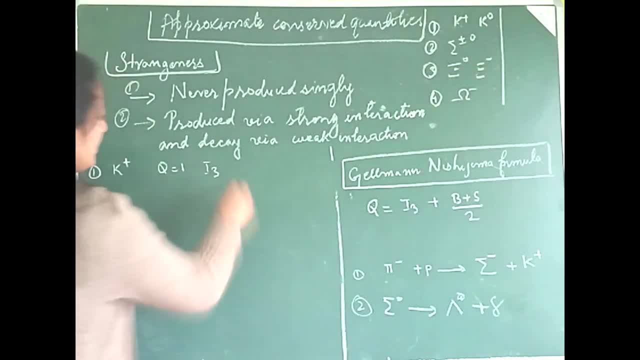 So doublet meaning your isospin is going to be half right. So now my I3 value will be plus half because this is with the higher charge right. So I discussed this in your isospin lectures. 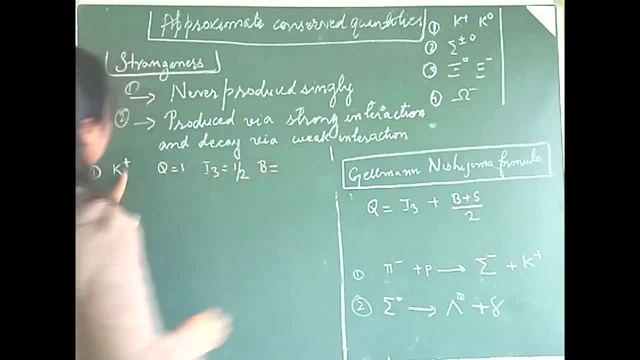 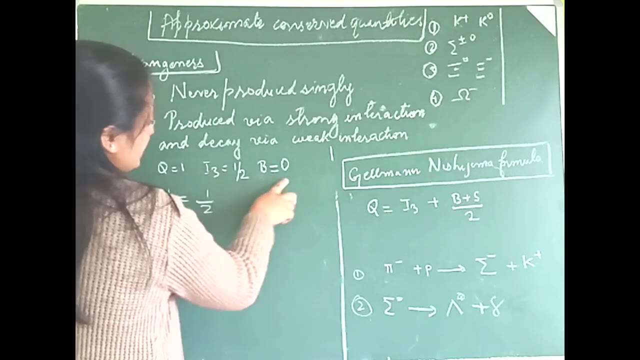 Now your B value. This is a meson, right. So Qons, they are mesons, Hence your barrier number is 0 here. So now, making use of this formula, making use of these quantities here, I get 1 equals to half plus this is 0.. 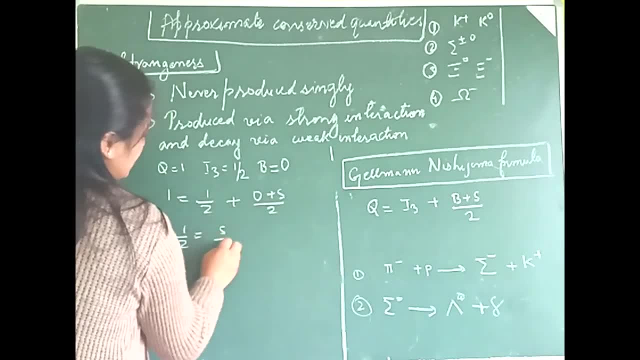 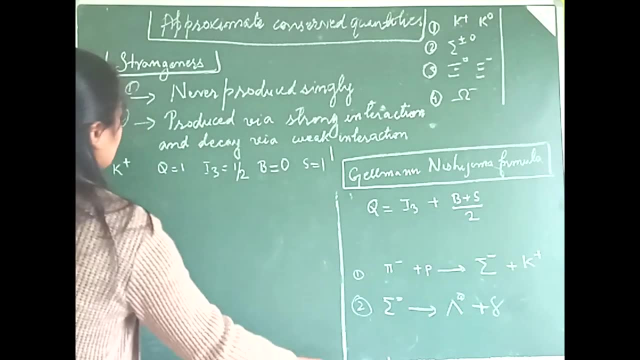 So S by 2.. So that gives me half equals to S by 2.. S is equals to 1, right, So S equals to 1. for your K plus Now for K minus, you get Q equals to minus 1.. 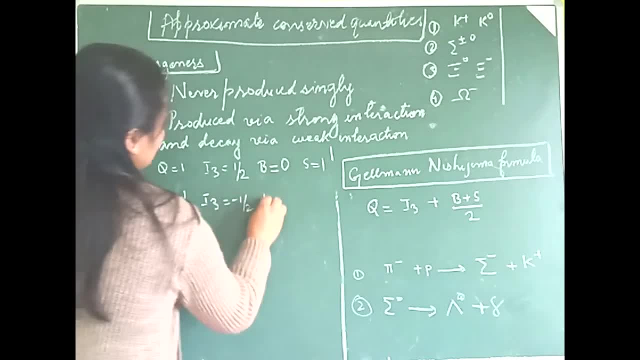 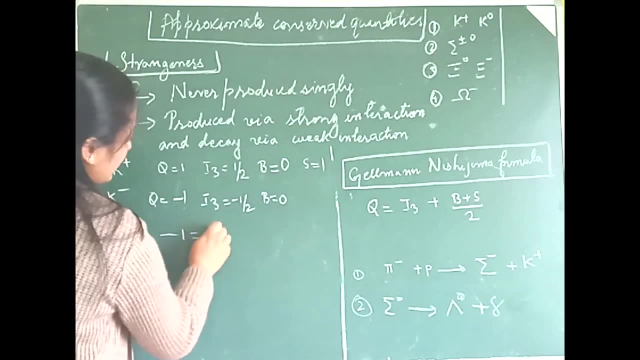 My I3 is minus half. Again, it is a meson, Hence your barrier number is 0.. Now, making use of this, I get: minus 1 equals to minus. okay, that is not K minus, That is actually K0.. 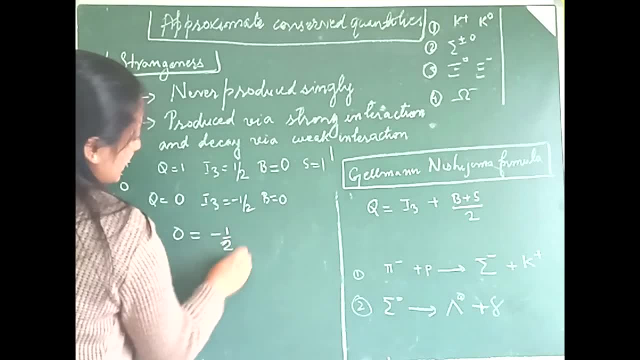 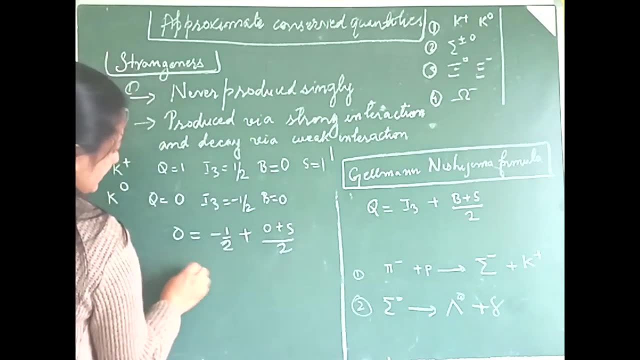 So hence it is 0.. So it is minus half, plus your B is 0, plus S by 2.. Again your S is 1.. So for this particle also, your strangeness is 1.. Now let us do for your another example, which say: is your omega minus, for which your Q is minus 1.. 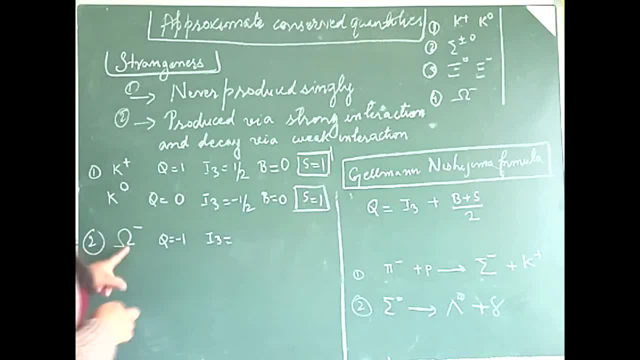 Your I3, remember this: omega is a single member in your family, right, So it is a singlet. I is 0. Hence your I3 is also 0.. So my B here, and because it is a baryon. 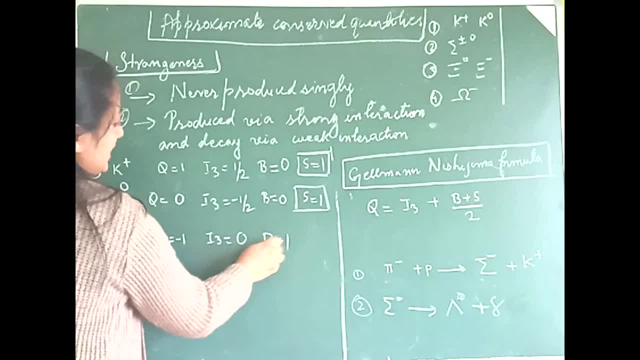 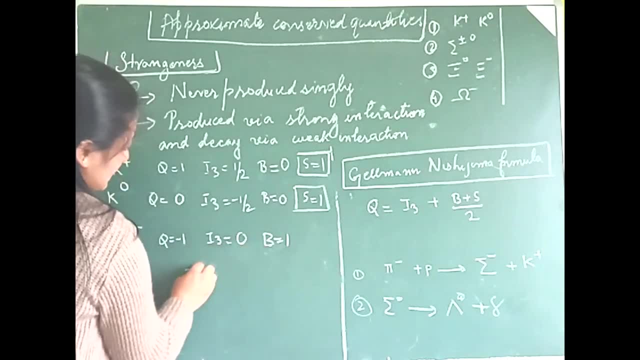 So all baryons, they have my barrier number as 1.. So I get my S using this formula as minus 1 equals to your 0. Plus 1 plus S by 2. So that gives me minus 2 equals to S plus 1, right. 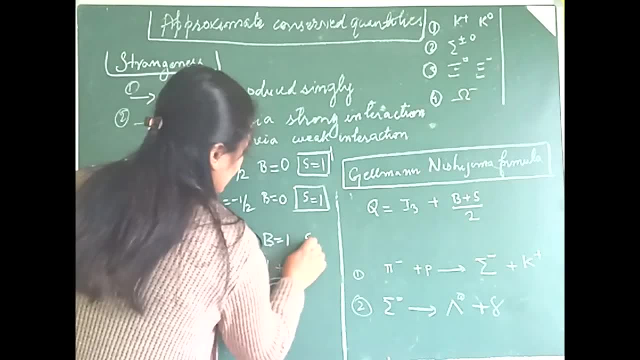 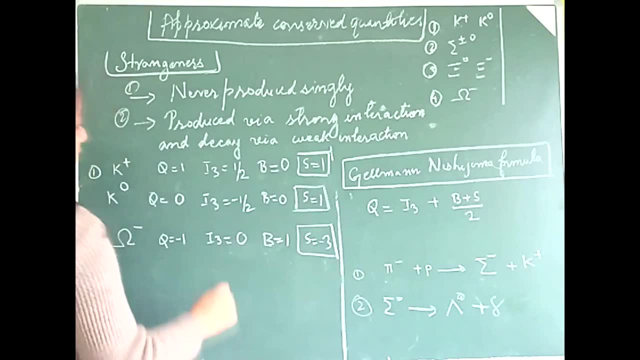 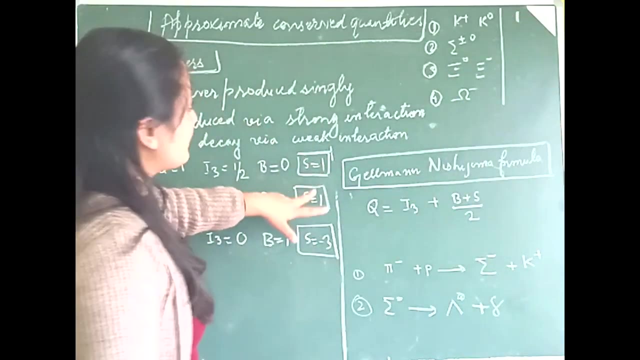 So it is S equals to minus 3.. So for this omega minus it is S equals to minus 3.. So similarly you can do for the others also. So you will see that for K plus K minus, your both strangeness value is 1.. 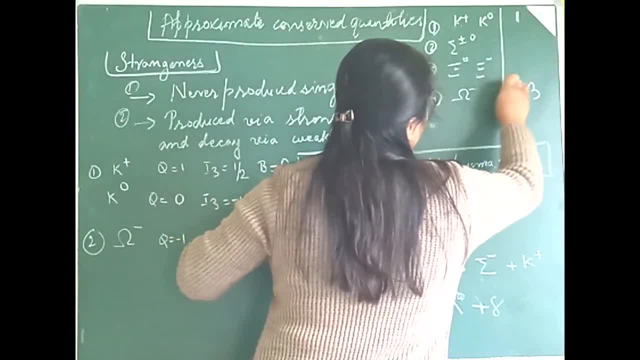 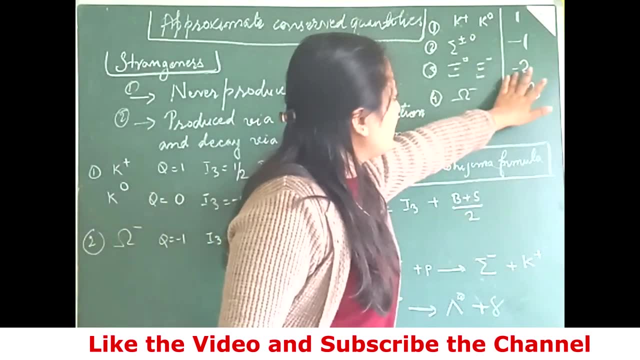 And for your omega minus, it is minus 3.. This is minus 1.. So this 2 you can take it as your home assignment, Where it is your minus 1, minus 2, right? So you are going to get minus 1 and minus 2 for the whole family. 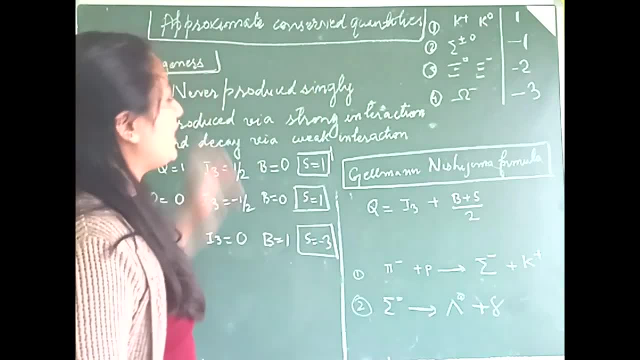 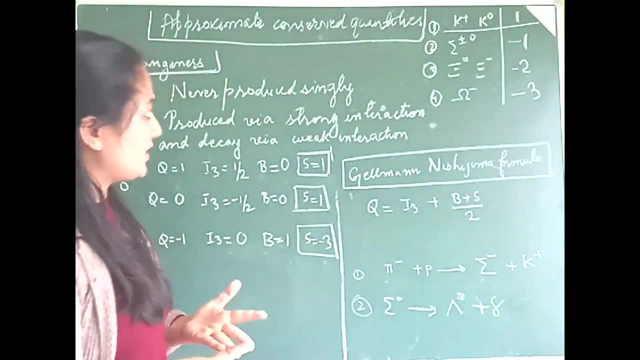 And minus 3 for your omega minus. So one thing I want to make clear here is for Kons- my strangeness- is positive, Whereas when I am talking about my hybrons, these are not hybrons, It is negative, right. 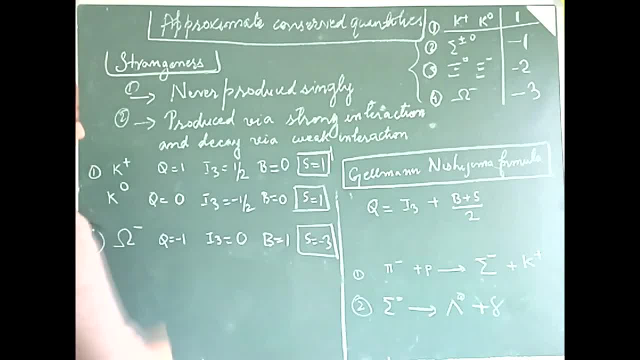 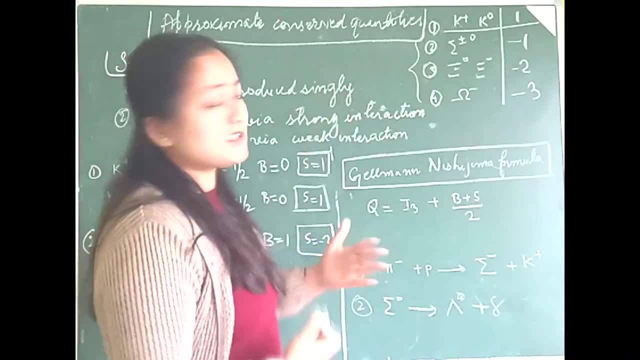 And strangeness: for all non-strange particles like your proton, your neutrons, it is all 0.. And for strange particles it is non-zero. It is either 1, minus 1, minus 2.. Such values right. 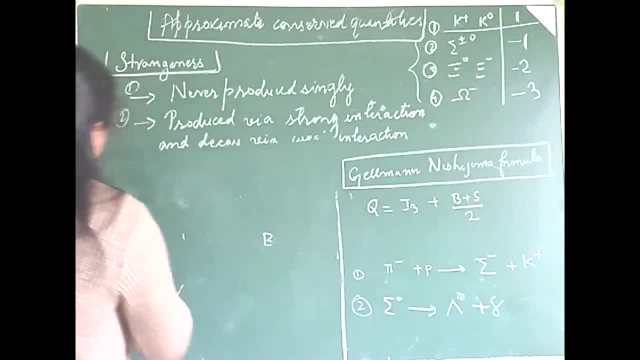 Now. so, having said that, let me also check, Like where all these S is conserved, right? So which are the interactions in which this S is going to be conserved? So first you have strong interactions, Then you have electromagnetic and you have your weak interaction. 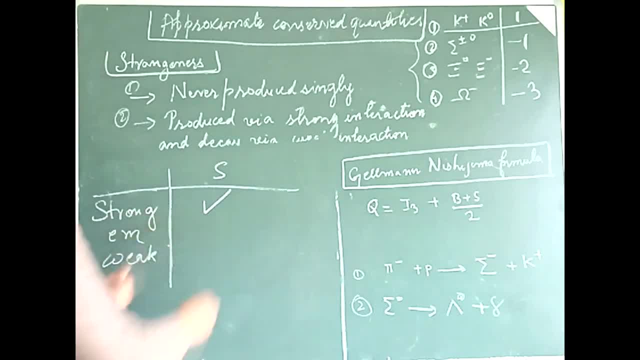 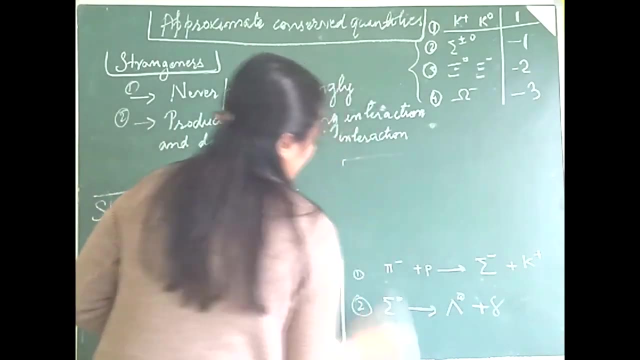 So your S is conserved in your strong interaction and your electromagnetic interaction, But it is not conserved in your weak interaction. So this is something which we must keep in mind, And let me give you one example. This helps me solving. 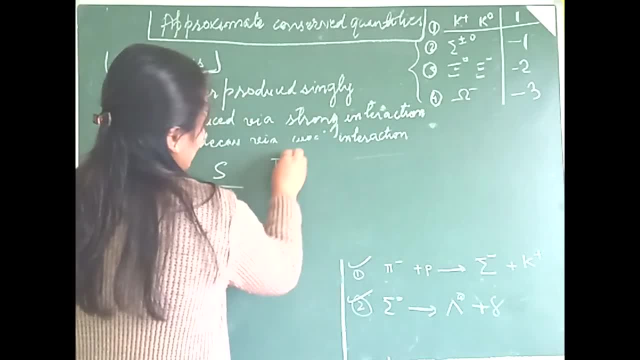 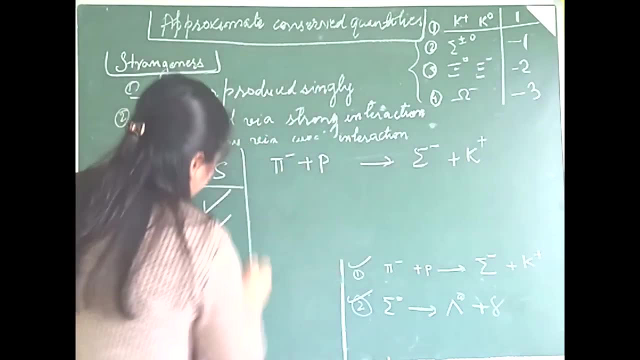 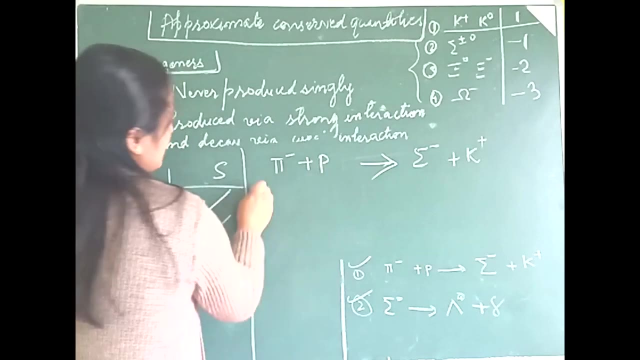 This you can take it as home assignment. Where your pi minus the first one is P, goes to omega minus plus K plus. Let us check whether this, I mean which kind of interaction, this particular interaction is. So let me check S. 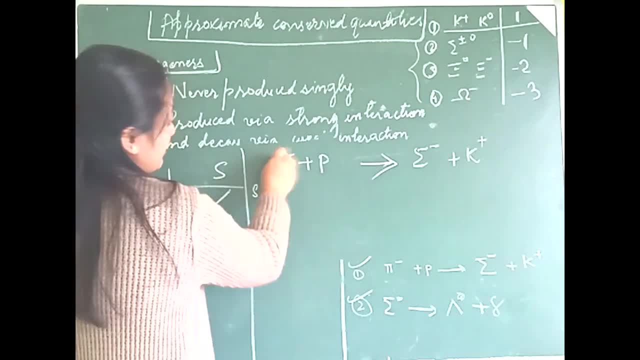 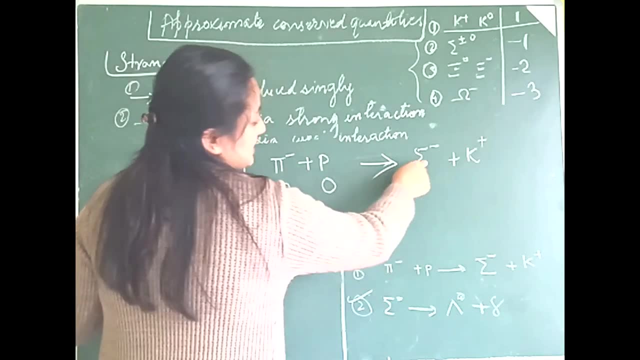 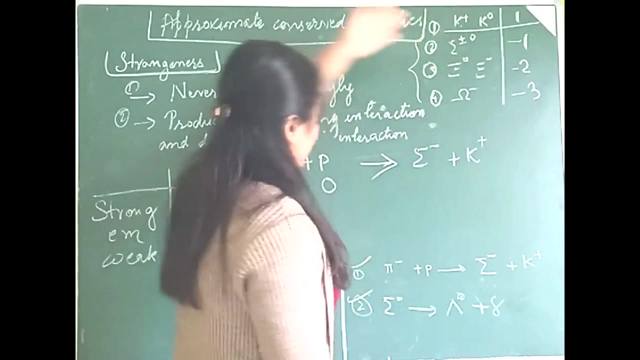 So S here is. so I am talking about strangeness, right, And this is: these are not strange particles. So 0, 0.. This is sigma, So sigma minus, sigma plus, sigma minus and sigma 0 is going to have my strangeness value as minus 1.. 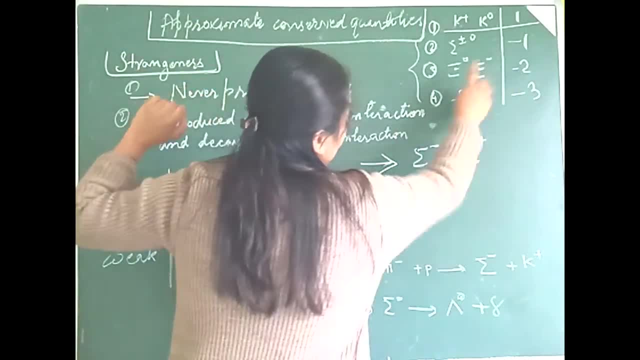 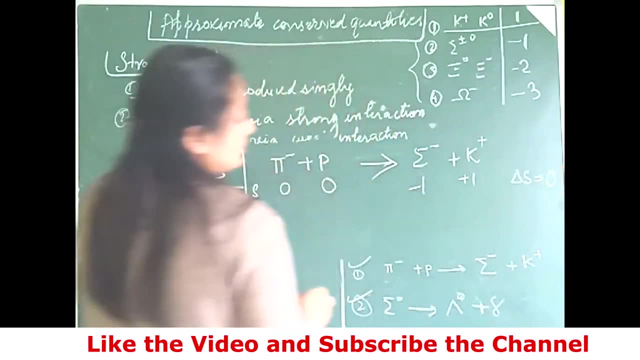 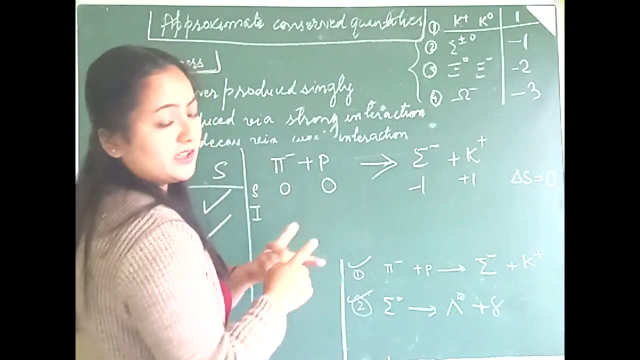 Hence this is minus 1.. My K plus is having plus 1.. So here I see, my delta S is 0, right, So that means my strangeness is conserved. Let me check my I. So I so this pions. they are 3 numbers in a particular. I mean there are 3 members in this pion family. So my isospin is 1.. Proton: there are 2 members and their it is given by half. Their isospin is given by half Sigma minus so 3 members again, So 1. K plus K plus 2 members in the family isospin 1.. 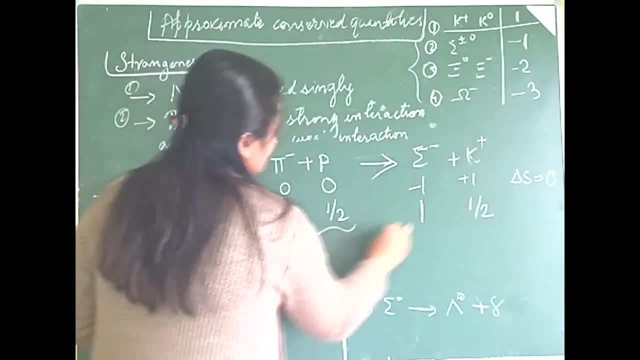 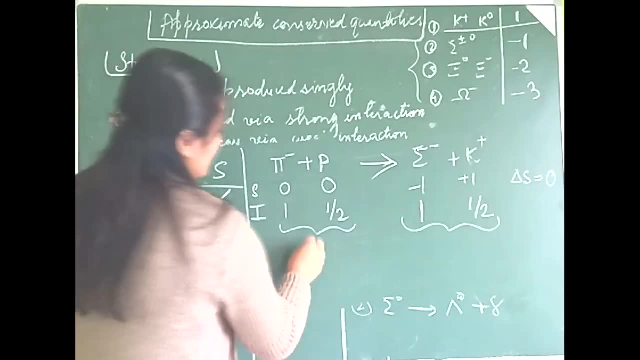 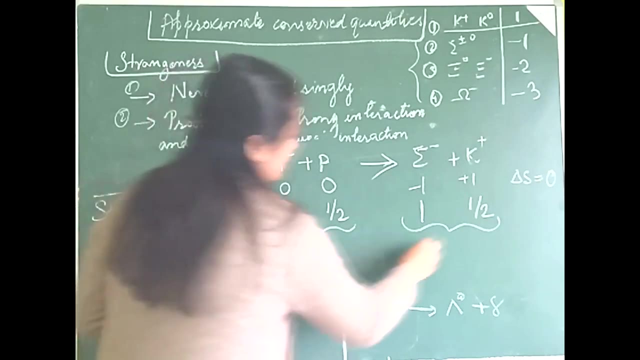 So these things I have mentioned clearly in your isospin video So you can follow that, So this. so my I is going to follow your vector addition. So it is going to be 1 plus half. If you do it, it is going to be 3 by 2, half by 3 by 2.. 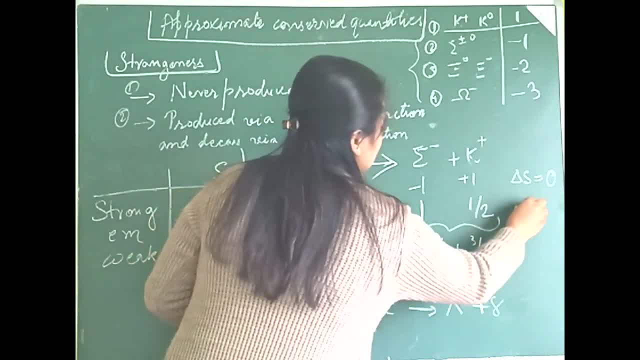 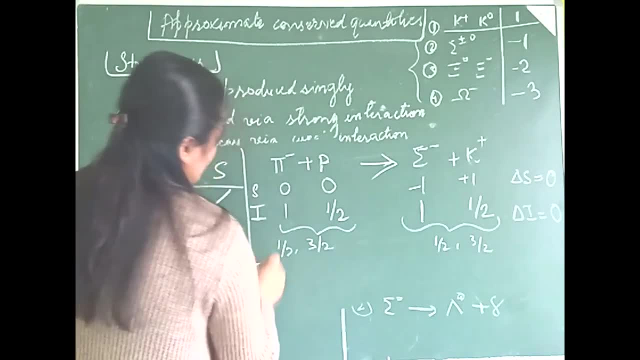 Again, it is going to be half by 3 by 2.. So my delta iron end is 0, right? So let me check my I3.. So my I3, this is pi minus 1.. So this is minus 1.. 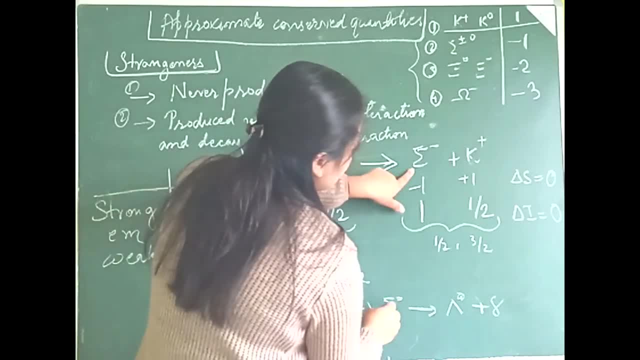 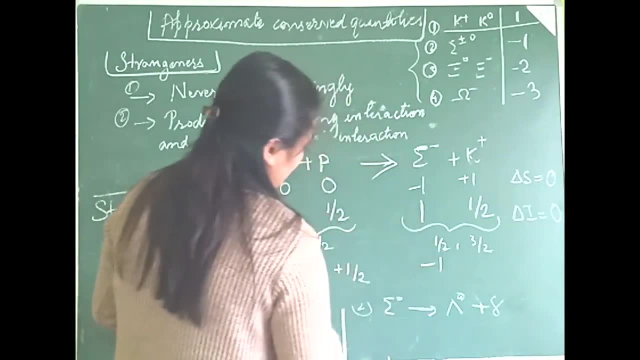 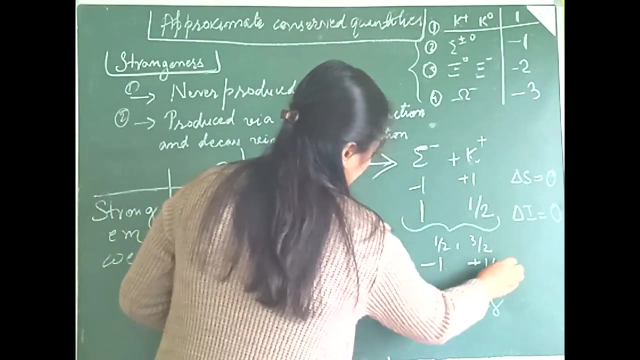 So proton is plus, half Sigma minus, so my I is 1 and this is sigma minus, So it should be minus 1.. And it is K plus and it is half I, So it is going to be plus half, right. 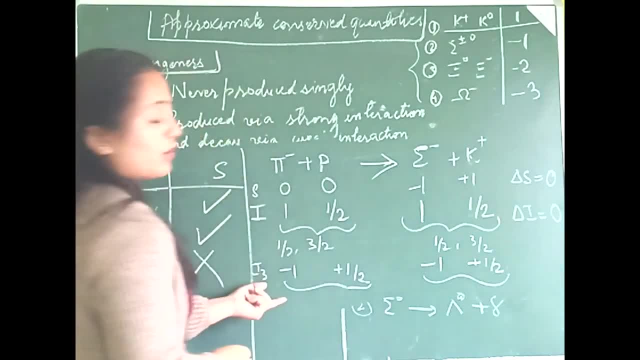 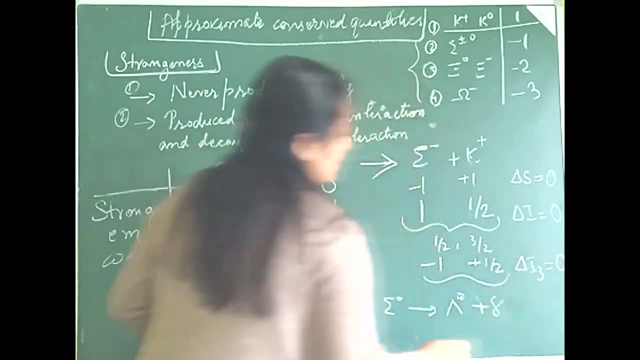 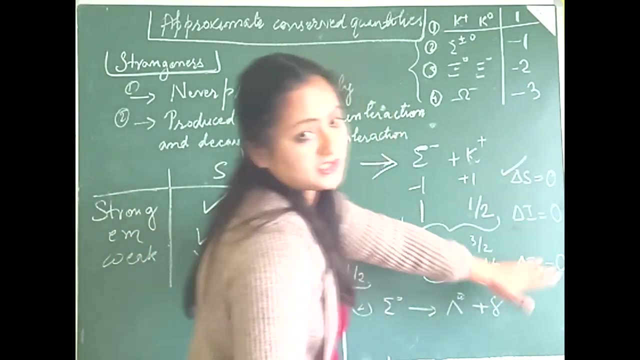 So again I see here. So I3 follows your algebraic laws of your addition. So I3. again, here is your 0. Hence we see that delta S is conserved, I is conserved, I3 is conserved. 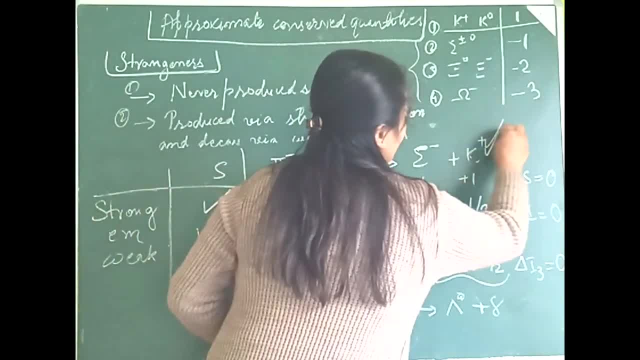 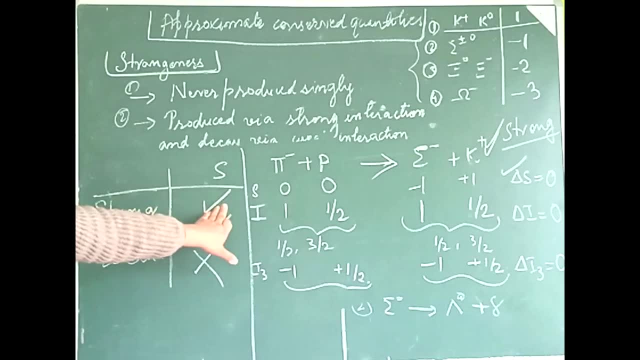 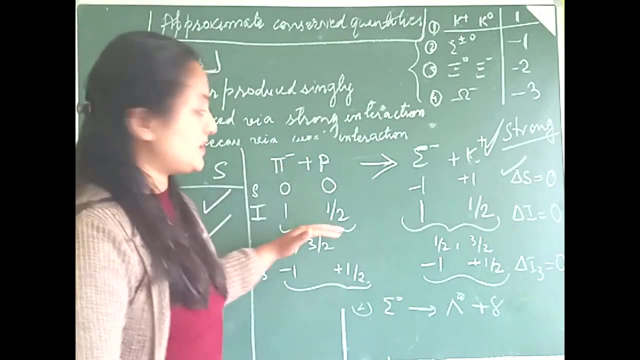 So basically meaning that the interaction which we are talking about here is strong interaction, because in strong interaction S is conserved And if you can recall your isosceles lectures there, I have said that I and I3 is conserved in both of your strong interactions, right? 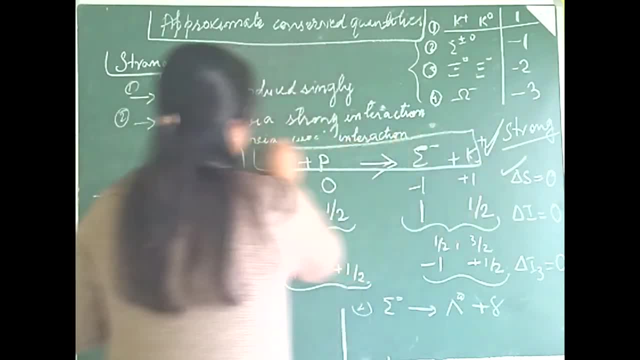 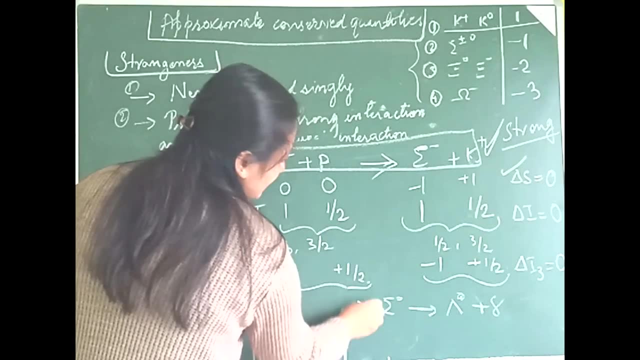 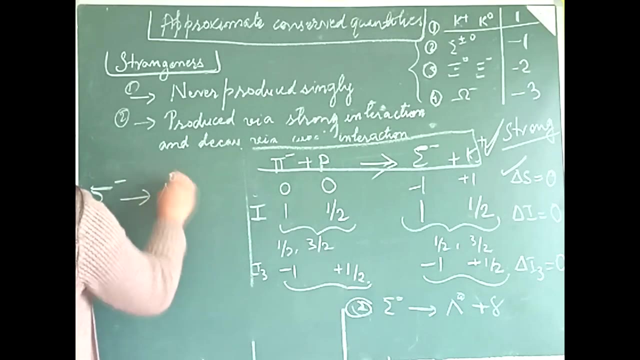 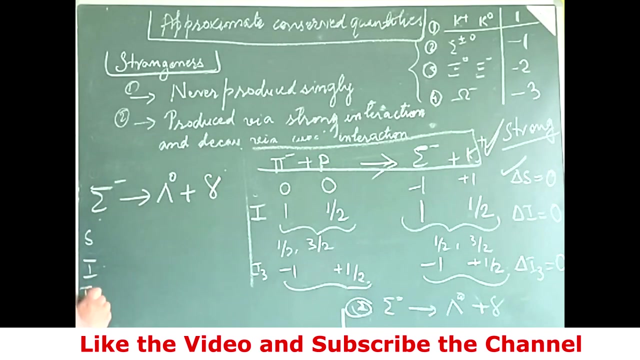 So, hence, this particular interaction is your strong interaction. So now, similarly, for this particular one, for 2, that is, your omega, sigma minus going to lambda 0 plus gamma, What you can do is you can check your S, you can check your I, you can also check your I3. 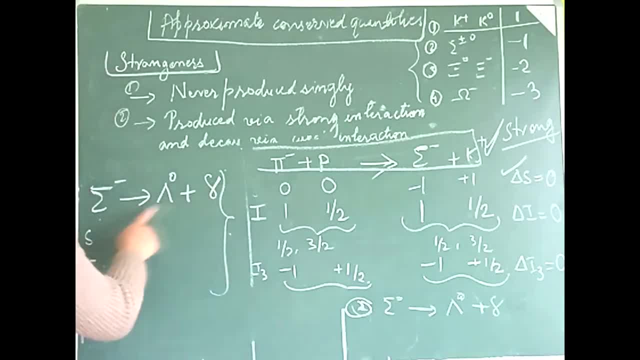 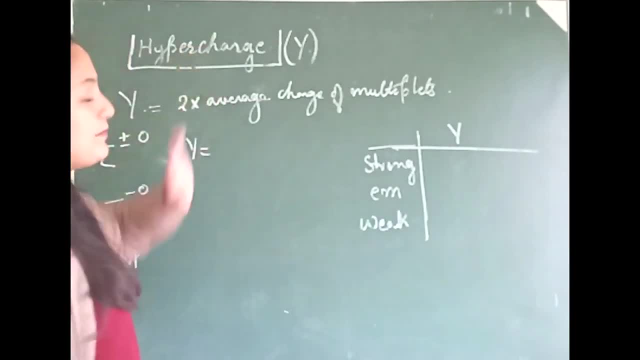 and then tell me which interaction. this is right. Okay, So another approximate conserved quantity is your hypercharge. Now, this hypercharge is also conserved in certain interactions and it is not conserved in some other interactions. So it is denoted by the letter capital Y and it is given by 2 times the average charge. 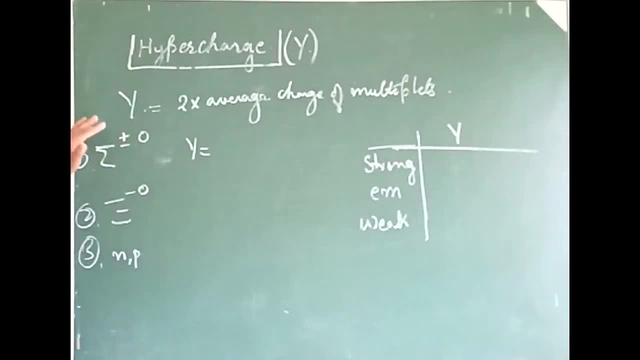 of the multiplex right. Okay, So let me calculate hypercharge for these 3 particles. So sigmas, cascades and your neutrons. okay, So Y is 2 times now it is written- average charge of the multiplex right. 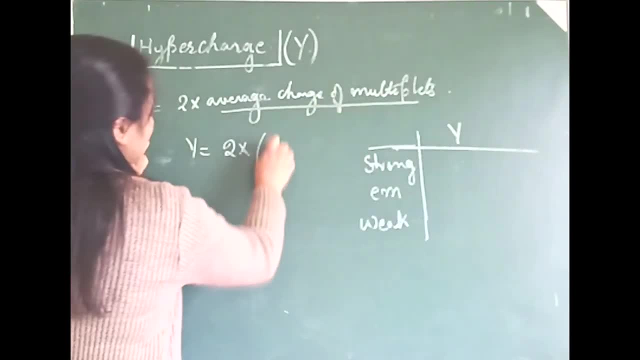 The charge is plus 1, minus 1 and 0.. So that basically meaning plus 1, minus 1.. So, divided by 3, right, So this is 0,. okay, Because 0,, so this is 0.. 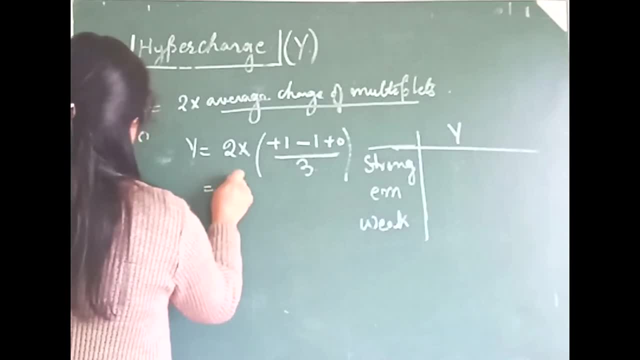 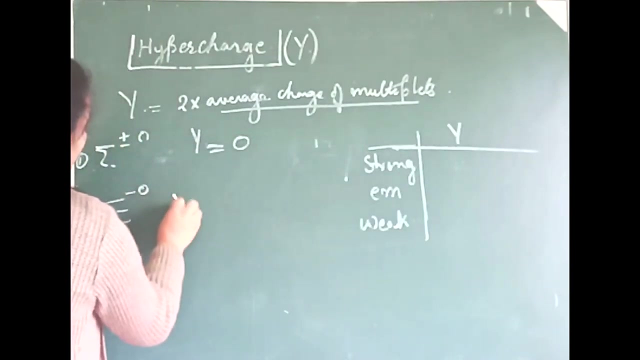 Now let me just write it here. So Y is 0.. Now Y here for your sigmas. it is 2 times the average charge of the multiplex, which is minus 1 plus 1.. Okay, So X is minus 0, divided by 2.. 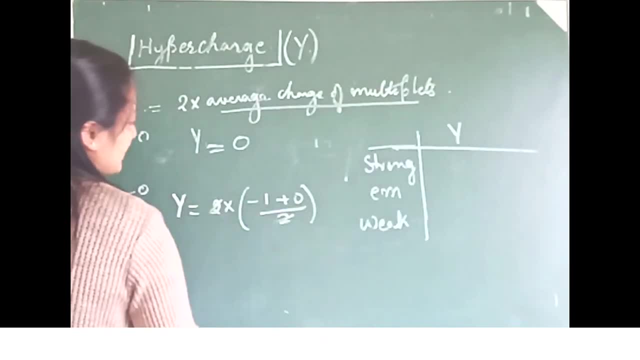 So this gets cancelled. So this means Y is minus 1 here. So the hypercharge is given by minus 1 here. Now for neutrons, so it is 2 into charge of neutron is 0 and that of proton is 1, means: 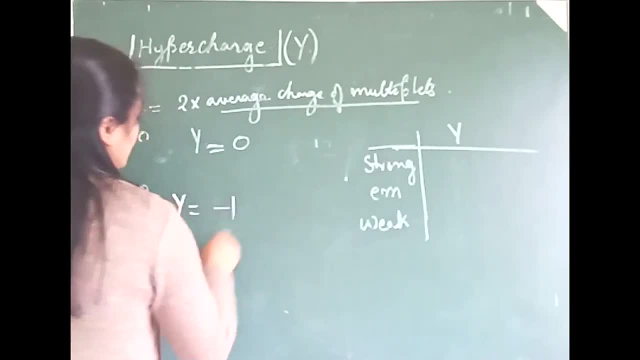 it is given by 1.. So the hypercharge for your neutrons is 1, right, Okay. Now this is considered as paper in this class. If you want, you can see the formula that we have here Now this hypercharge. it is conserved in your strong interaction, in your electromagnetic interaction, but it is not conserved in your weak interaction. okay, 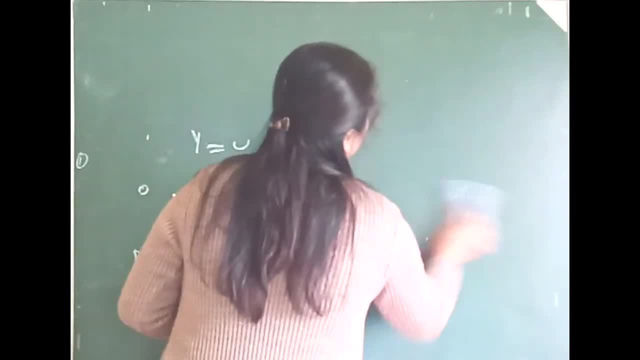 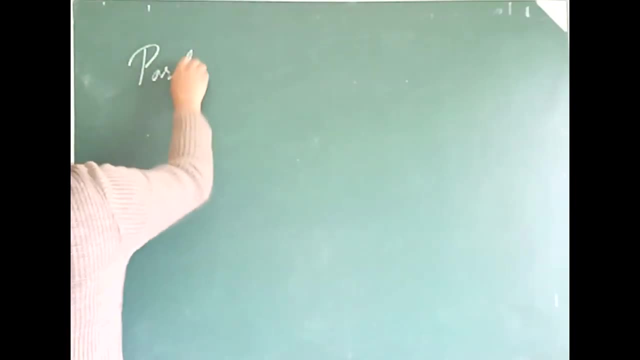 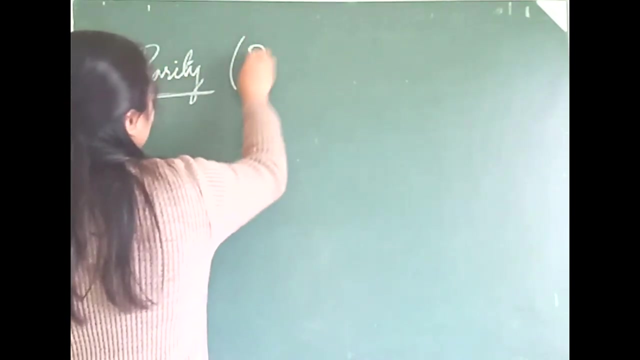 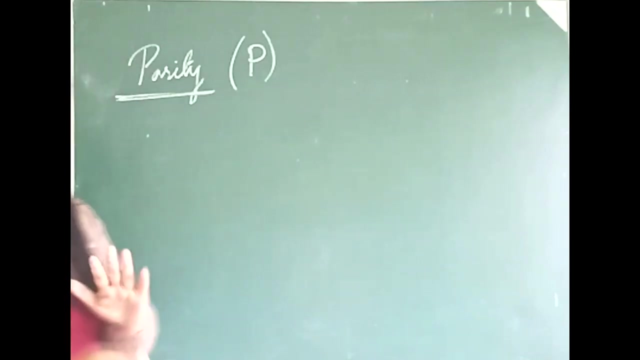 Now another quantity in your light-year hypercharge, which again is not your approximate, which again is your approximate- conserved quantity is parity, right. So parity is denoted by the capital P and this is actually your mirror symmetry, right? like when you take your space reversal. so that is your parity.